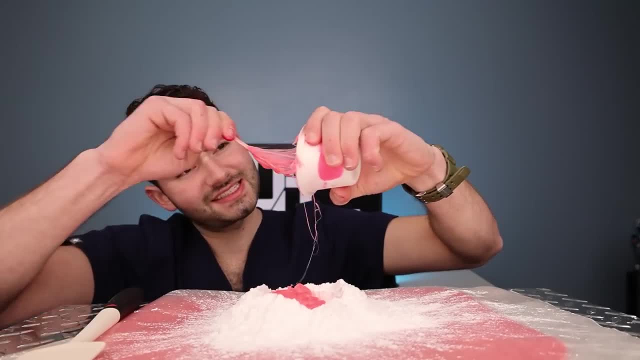 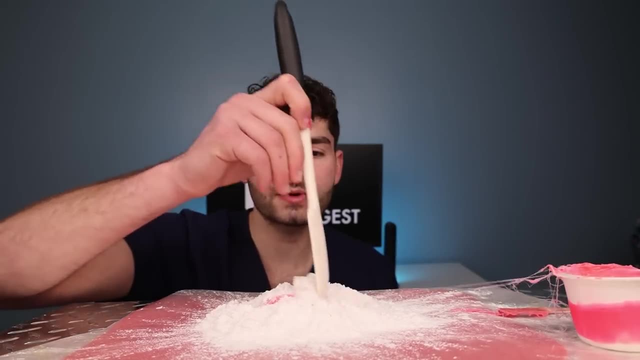 And then add the gum mix Fat glob, Get every single last drop of the gum into the center. Oh, it's so good. It's so messy. Because it's hot, you're gonna fold it over and incorporate some of the powdered sugar until it's not too sticky. 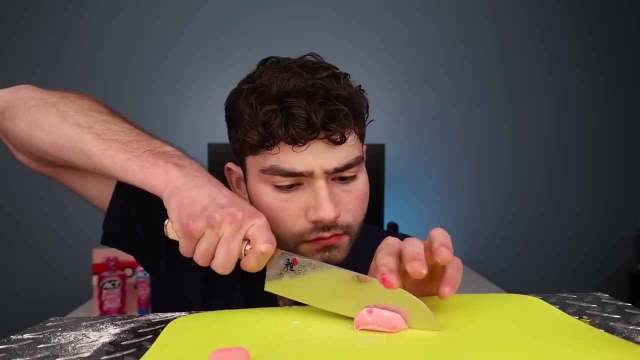 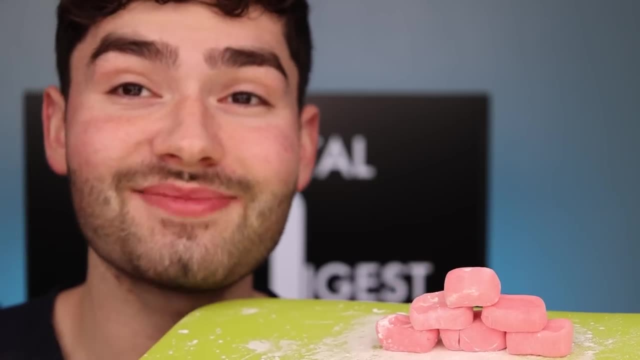 Smells delicious. Once it's got the right texture, it's time to make some cuts, Add a little bit of sugar and shape them to how you want it. I want little cubes like Hubba Bubba. Now that we got our gorgeous pieces of gum, let's test them out. 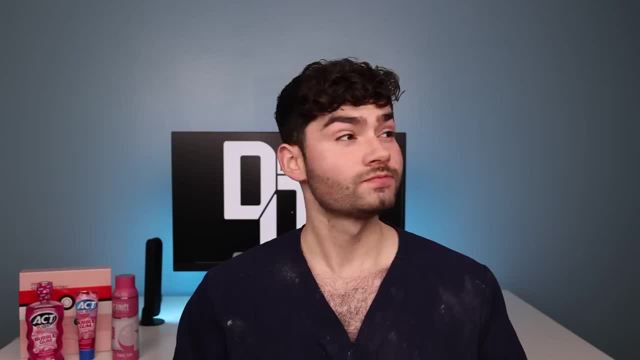 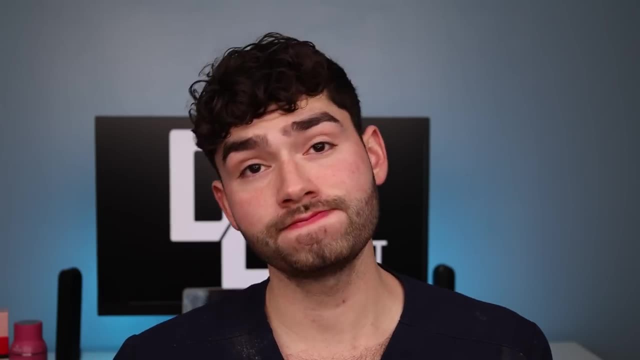 It's disclosing time. It's so soft. I think I might have added too much flavor, though I think my lips are getting more pink as I chew it. Let's see how big of a bubble I can blow. I think we need more gum. 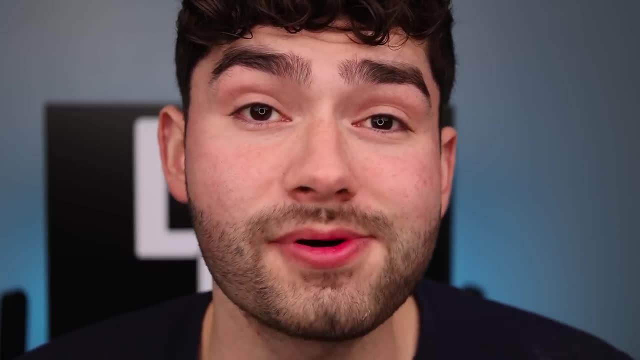 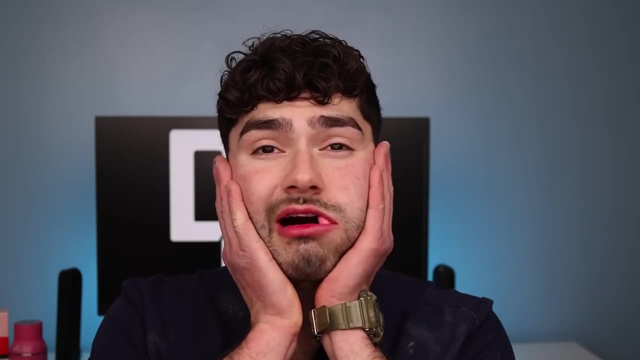 Oh yeah, My teeth are getting really pink after chewing this gum, but it tastes pretty good. I look like a chipmunk. Let's blow this bubble. I want it larger than my face. Why is it so hard? My jaw is hurting. 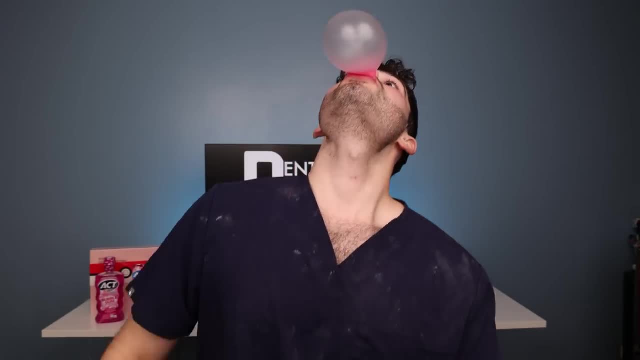 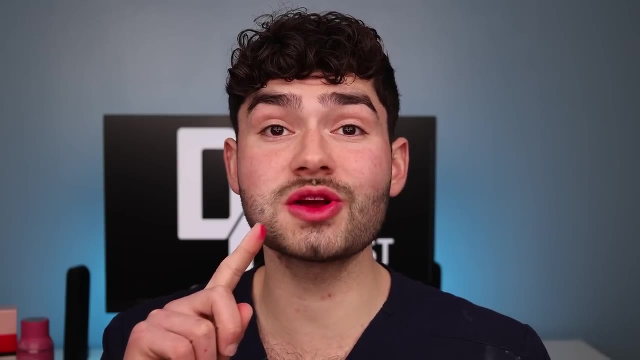 Oh, did you see that? That was huge. It's a pretty good bubble gum, but I think it's making my tongue pink. Oh no, This gum had lots of sugar, so let's see if it stained my teeth. Let's check the before results. 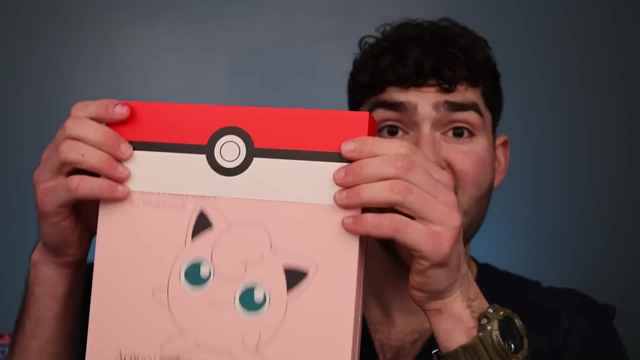 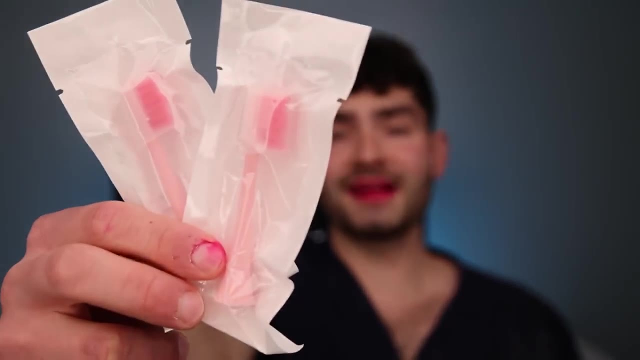 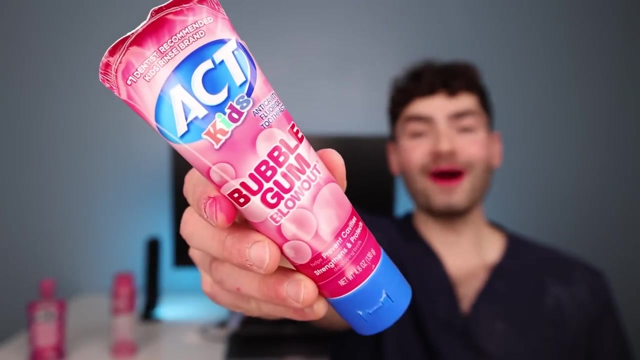 Jigglypuff Toothbrush- Yeet, It comes with a customizable charging base, two spare bristle heads and a Jigglypuff toothbrush. Let's check out the bristles on this toothbrush. Bubble Gum, Blowout Toothpaste. 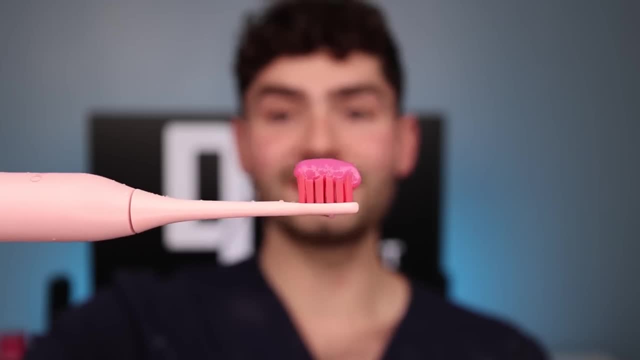 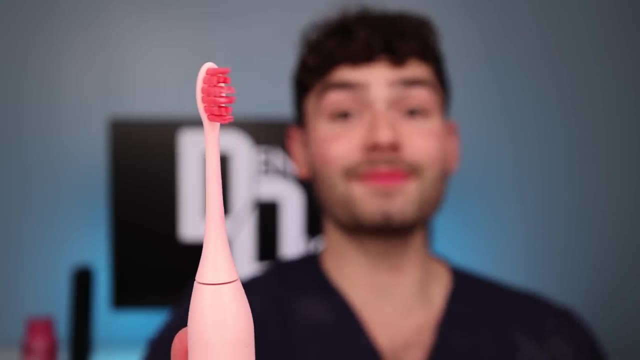 Fat Gloss. This is Dental Digest. Let's get brushing. This toothpaste tastes like Hubba Bubba and this toothbrush is Hubba Hubba. These sonic vibrations are tickling me. It's tickling my teeth, but it tastes delicious. 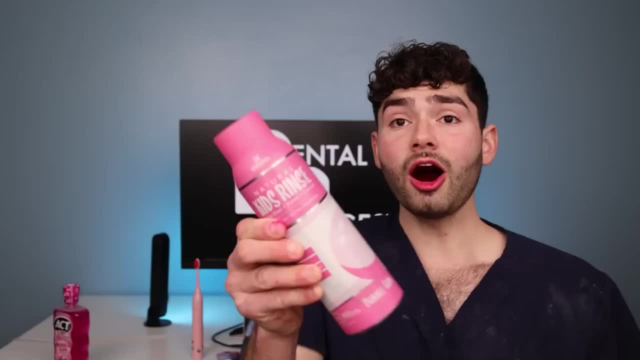 Bubble Gum Mouthwash. Let's see which one tastes better, The all-natural or cavity protection. Up first the all-natural. Why is it so dusty? Ugh, I think this stuff stinks. It's not expired, It just stinks. 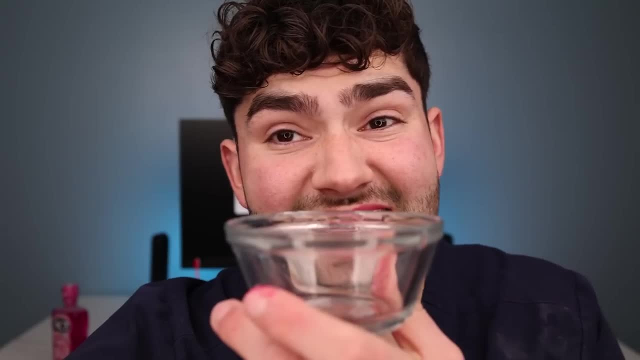 Let's see what it looks like. Oh what? Why does Bubble Gum Mouthwash look like pee pee? I don't think I can drink this. This is Dental Digest. You guys better subscribe to this channel, because I'm about to drink mouthwash that. 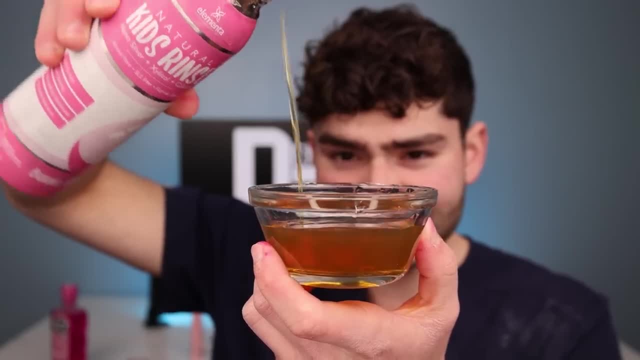 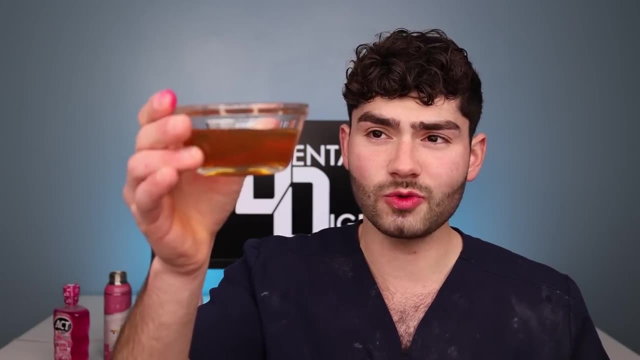 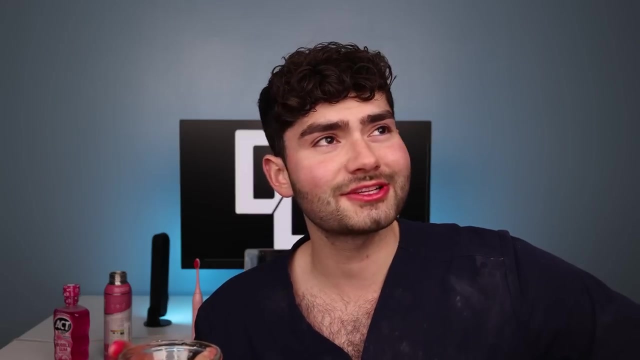